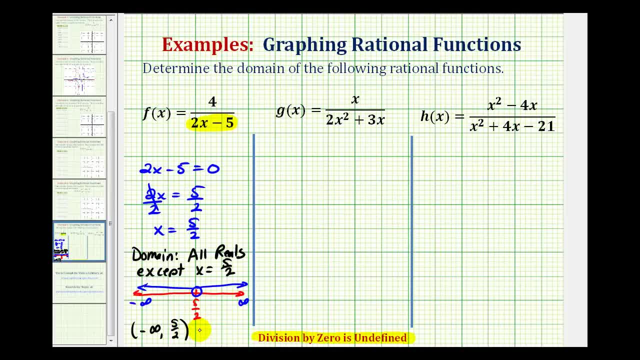 to five halves union, five halves to positive infinity. So here we express the domain in words, Here we express it as a graph And here we express it using interval notation. For our second function, we need to set two x squared plus three x equal to zero. 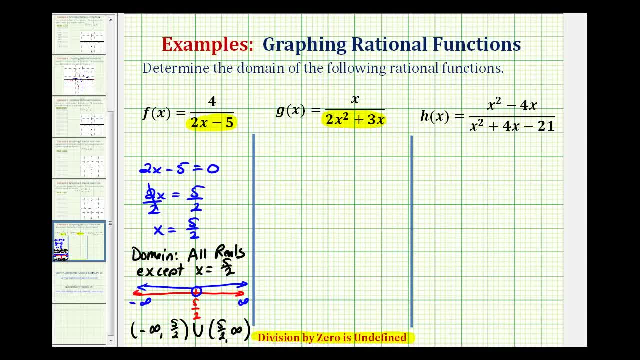 and solve for x to determine the excluded values. So we'd have the equation two x squared plus three x equals zero. First step in factoring is to factor out the greatest common factor, which is x. So we have x times the quantity two x plus three. 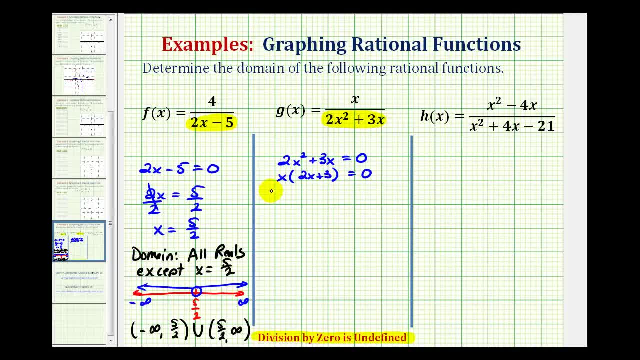 Equals zero. So either x equals zero from this first factor, or two x plus three equals zero. Well, here we would subtract three and divide by two, so we'd have x equals negative three halves. So we must exclude zero and negative three halves from the domain. 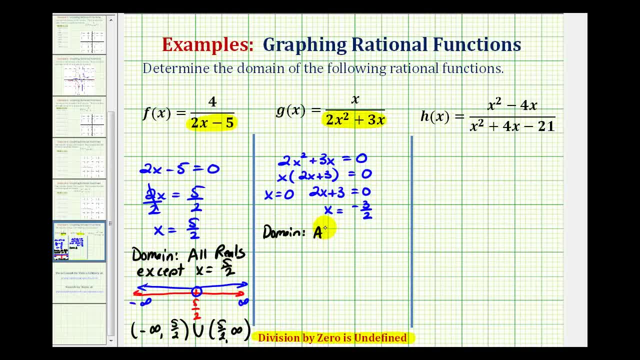 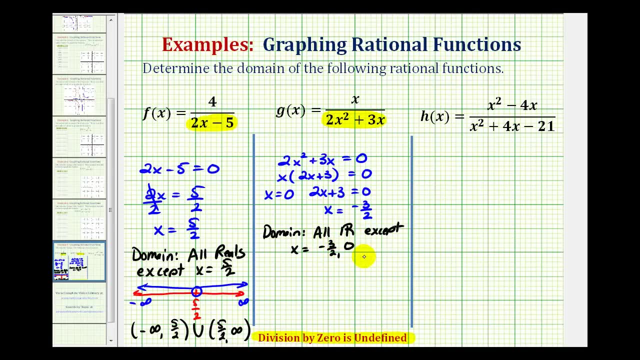 So the domain would be all real numbers. We can abbreviate real numbers by using this symbol: here, Two legged r except x equals negative three halves and zero. So again, if we wanted to graph the domain, we would sketch a number line. 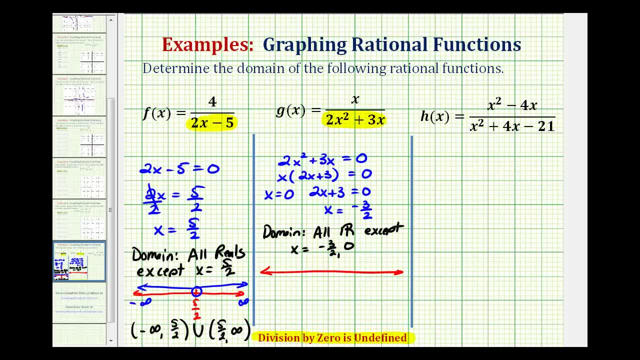 and exclude zero and negative three halves. So let's say zero's here and negative three halves is here. We'd exclude these two values and graph every other real number. So we'd graph in between, to the right and to the left. 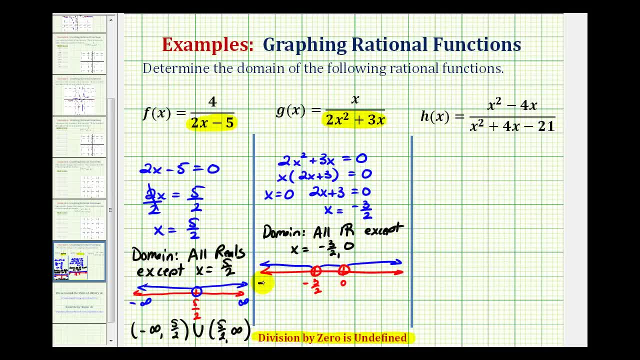 So if we wanted to express this using interval notation, this would be negative infinity, this would be positive infinity. So we'd have, from negative infinity to negative, three halves union from negative three halves to zero, union from zero to infinity. And then, for the last example, 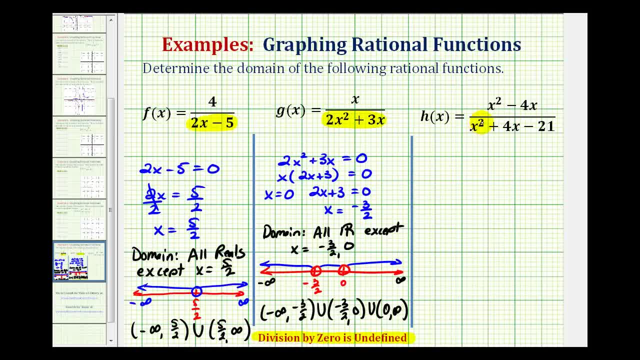 we'd take the denominator of x squared plus four, x minus twenty one, equal to zero, and solve for x to determine the excluded values. So we'd have x squared plus four, x minus twenty one equals zero. This does factor, So the first terms would be the factors of x squared. 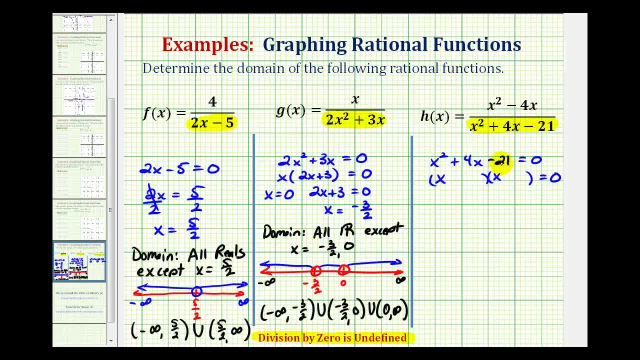 which would be x and x. Now we want the factors of negative twenty one that add to positive four, So that would be positive seven and negative three. So the solutions to this equation are: x equals negative seven or x equals positive three, Which means these values make the denominator equal to zero. 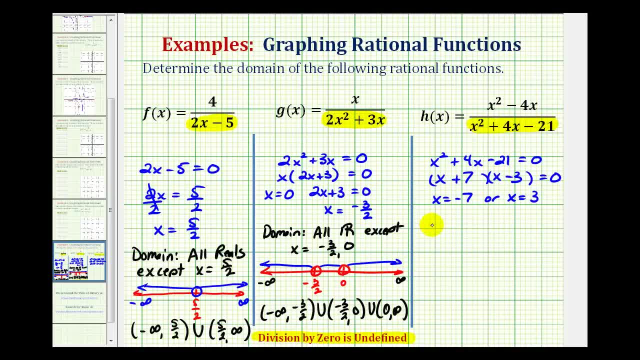 and must be excluded from the domain. So the domain would be all real numbers or all reals except x equals negative seven and three. We'll graph the domain as well. So we would plot: negative seven, positive three. exclude these values with open points. 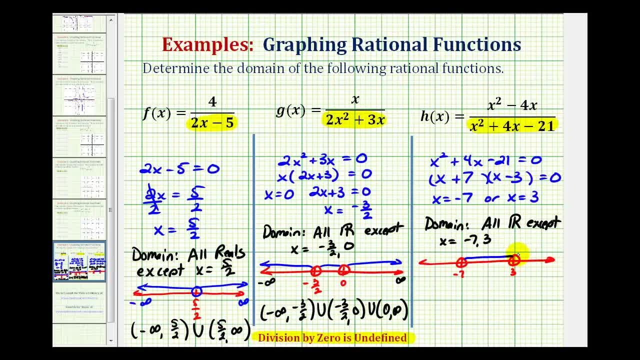 and graph every of the real numbers. So we graph in the middle, to the right and to the left. So using interval notation. on the left we'd have the interval from negative infinity to negative seven, Union negative seven to three. 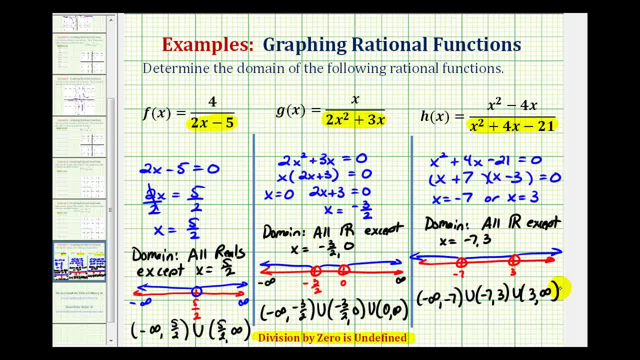 Union three to infinity. Now there is one more thing I'd like to mention. Sometimes rational functions will simplify because they have common factors between the numerators and denominators, But we do not want to simplify them before determining the domain and range. 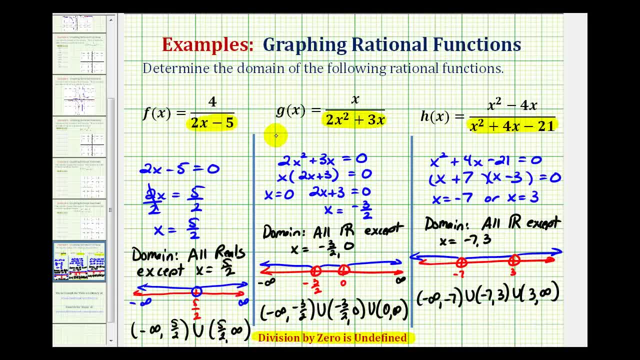 What I mean by that is, if we take a look at g of x, we could write this as: g of x equals the numerator of x, and the denominator in factor form would be x times the quantity two x plus three. 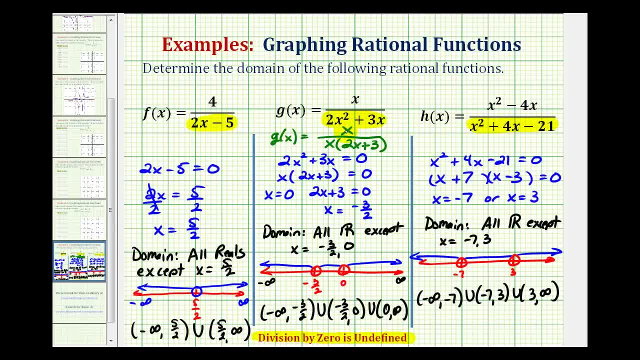 So we do not want to simplify out this common factor of x, because then we would not exclude zero from the domain. So this common factor does produce a hole in the function, while the zero of this factor produces a vertical asymptote, So it does affect the graph.